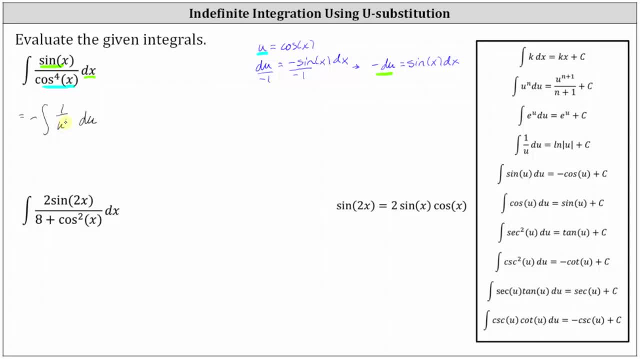 the integrand function is just one, divided by u to the fourth. Next, let's write this as negative, or the opposite of the integral of u to the power of negative four, du. and now we can apply the power rule of integration. The antiderivative is negative u to the power. 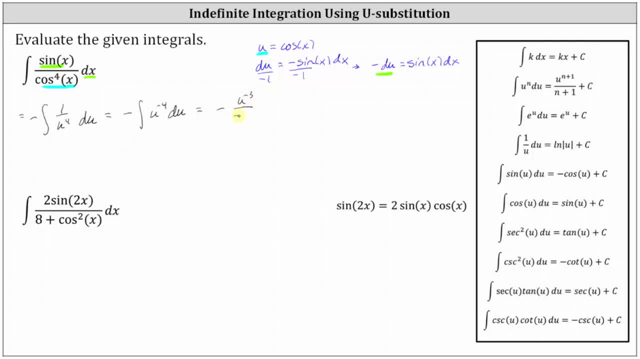 of negative four plus one which is negative three, divided by negative three plus c. Simplifying and writing in terms of x, we have positive 1, third and u to the power of negative three is really cosine x raised to the power of negative three. 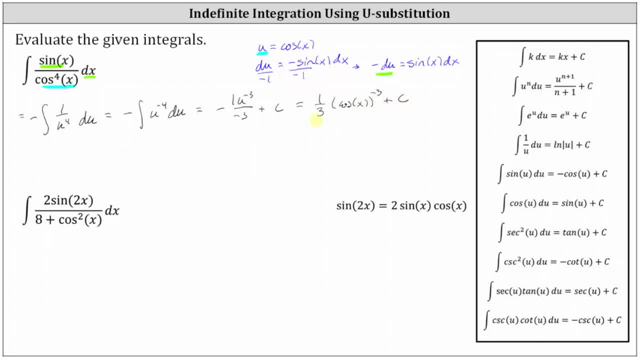 negative three plus c. Let's write this using a positive exponent: This is equal to one divided by the product of three and the cube of cosine x, or cosine cubed x plus c. Now let's write the antiderivative using big F of x, where big F of x is equal to again one divided by the product of. 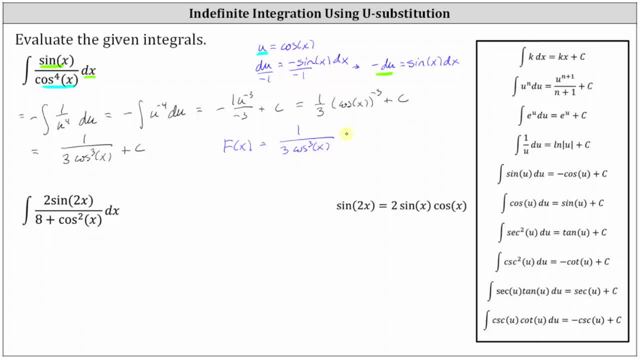 three and cosine cubed x plus c. This is the family of functions whose derivative is equal to the given integrand function. Looking at our second example, notice how we have a double angle in the numerator and a single angle in the denominator. Let's first perform a substitution. 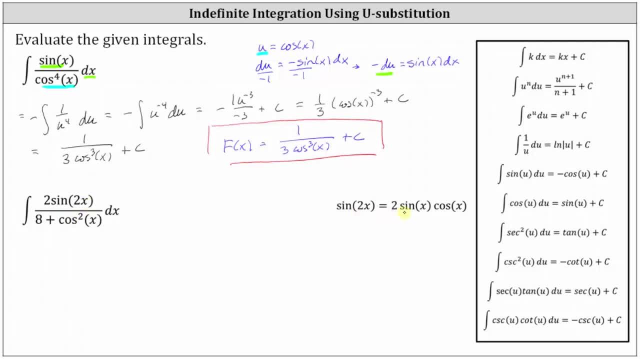 for sine 2x, where sine 2x is equal to two times sine x times cosine x and therefore we can write the numerator as two times two sine x. This gives us cosine x, which gives us four sine x times cosine x in the numerator. 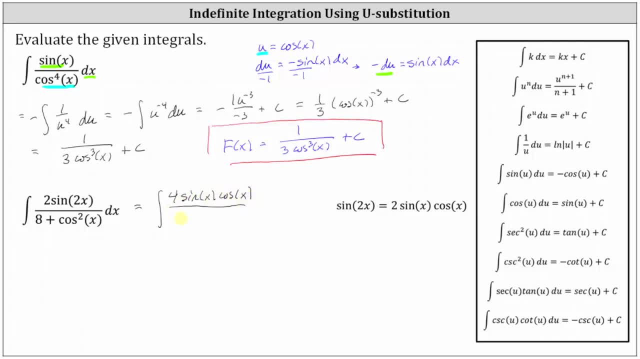 and the denominator remains eight plus cosine squared x. Now this one's a little bit tricky. From here, we're going to let u equal the denominator of eight plus cosine squared x, which I'm going to write as the square of cosine x. And now du is equal to the derivative of sine 2x. 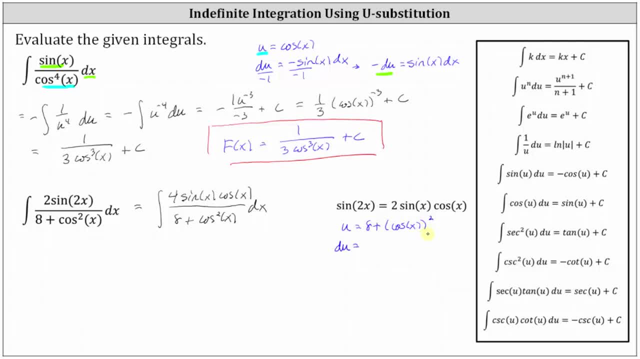 So we're going to write the derivative of eight plus the square of cosine x times dx, which is zero, plus two times cosine x to the first times, the derivative of cosine x, which is negative, sine x- Notice, here I'm applying the chain rule- and then times dx. 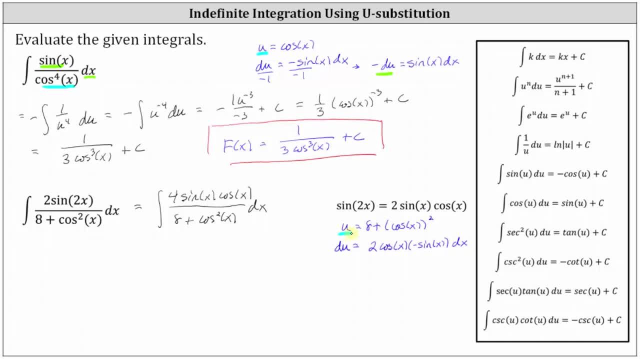 And now, looking back at the integral, since u is equal to eight plus the square of cosine x, we can write the denominator as u and we can see we're left with four sine x- cosine x- dx and we have du equals two cosine x times dx. 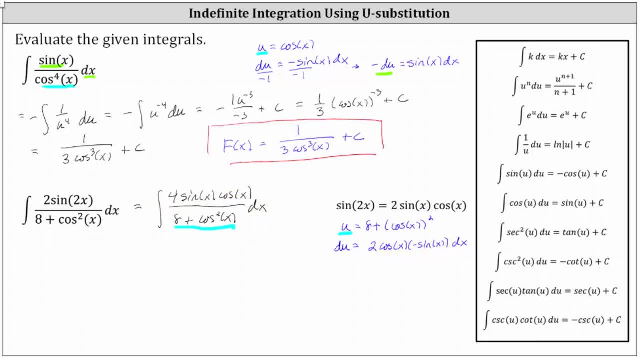 Let's first write this as du equals negative two: sine x, cosine x, dx. And here we have a choice: We can multiply both sides by negative two, so that the right side matches what we have in the integral, or we can just solve for sine x, cosine x, dx. 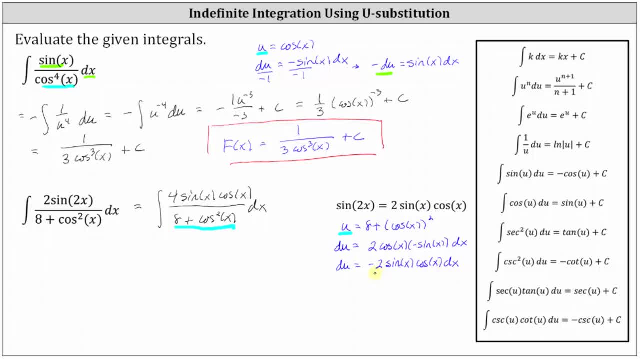 I'm going to be consistent and solve for sine x- cosine x dx by dividing both sides by negative two, which means negative one half du is equal to sine x times cosine x dx. So now we can substitute negative one half du for sine x- cosine x dx and factor out the four. 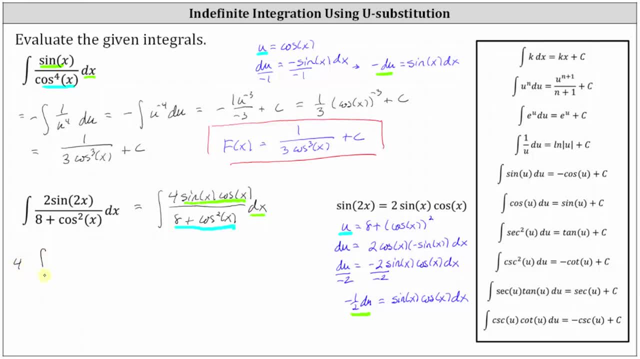 So, writing in terms of u, we factor out the four, and then again, sine x, cosine x, dx is negative one half du. So we'll factor out the negative one half and then we have du. and since the denominator is now u, the integrated function is just one divided by u. 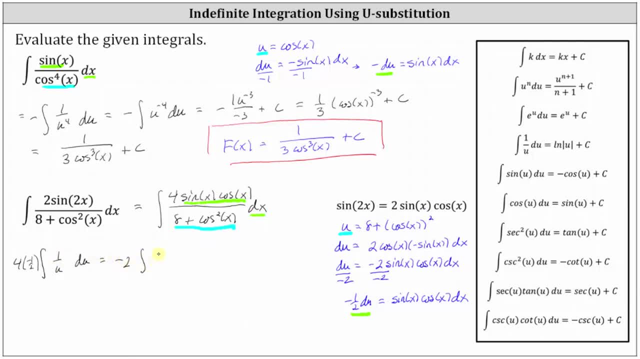 Simplifying, we have negative two times the integral of one divided by u du, and the integral of one divided by u du equals natural log absolute value of u plus c, which in our case gives us negative two times natural log absolute value of u plus c. 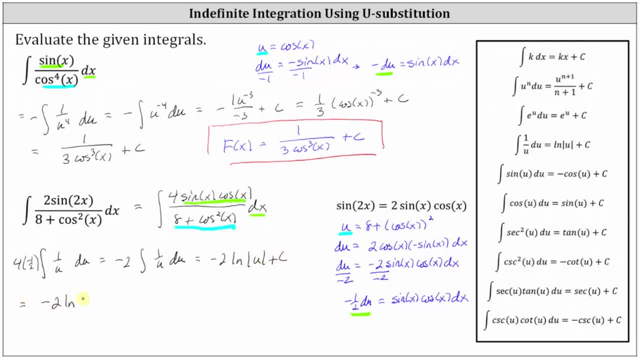 which in terms of x, is negative. two natural log absolute value of eight plus the square of cosine x, or eight Plus cosine squared x plus c, And again we can label this big F of x. We can actually also drop the absolute value here. 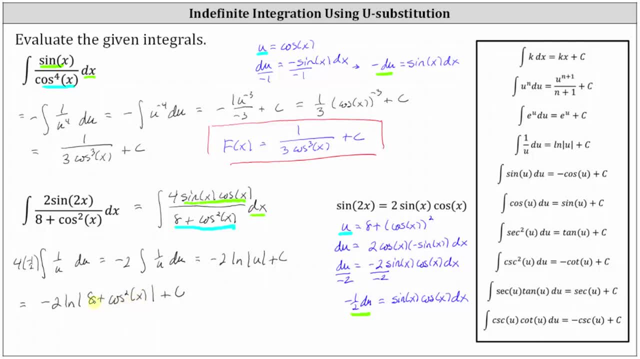 because cosine squared x is always positive and eight is also positive, which means we can write big F of x, as big F of x equals negative, two times natural log of just the quantity eight plus cosine squared x plus c. It's not wrong to leave the absolute value, but in this case it's not required. I hope you found this helpful.